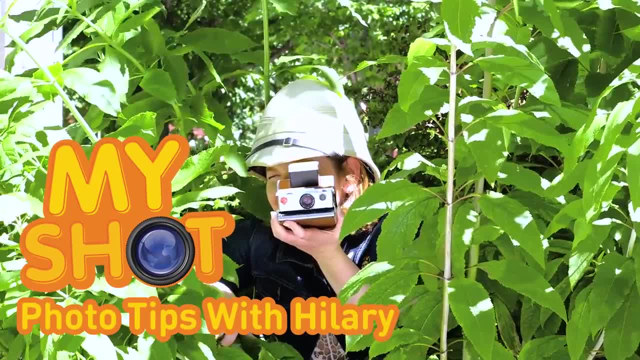 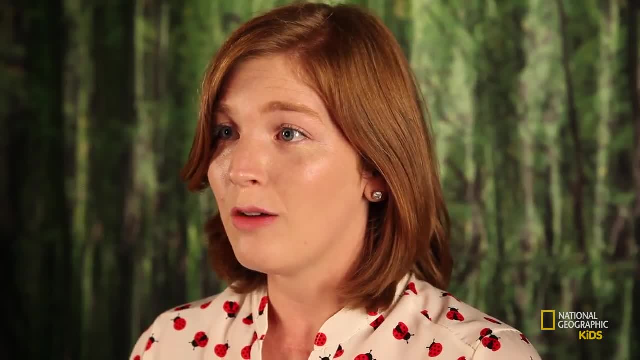 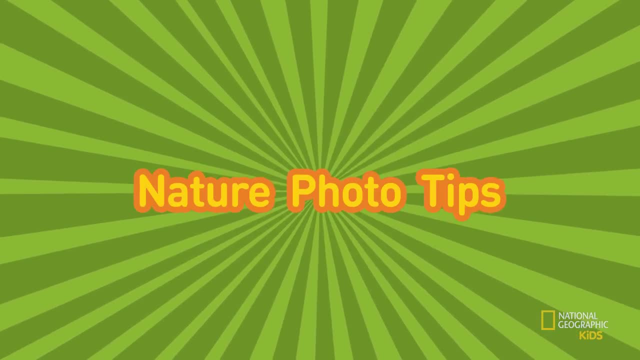 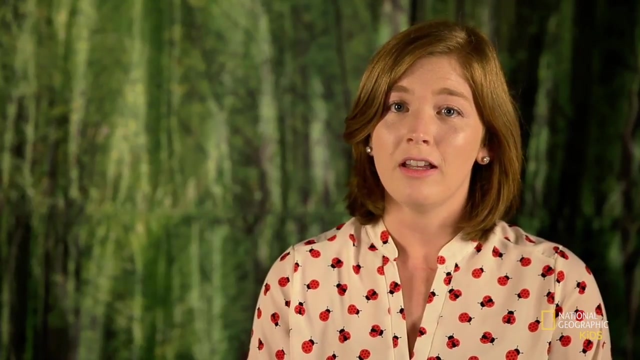 This is My Shot Photo Tips with Hilary and I'm Hilary. Grab your camera and head outside To help you get your best shot. we've asked professional wildlife photographer Gabby Salazar to share some of her secrets. Find a different perspective, Look for new and exciting ways to photograph your subject. 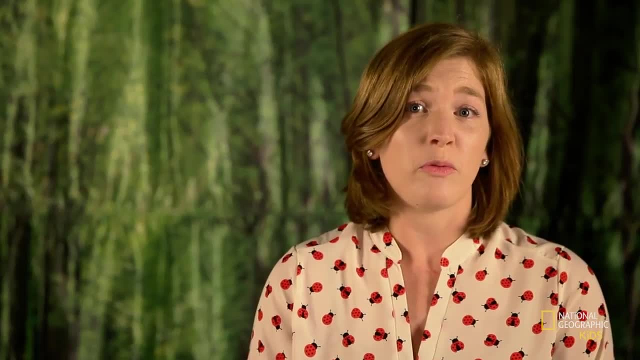 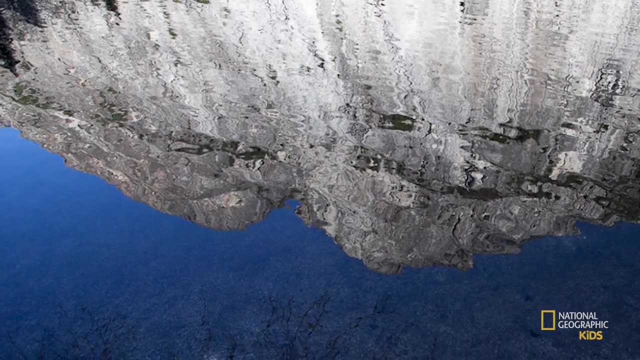 Look up and look down. You might not be able to move your subject, but you can move around it. Don't be afraid to get down on the ground for a new angle. Instead of taking a normal landscape photo of this mountain, Gabby decided to show it reflected in the river. The image: 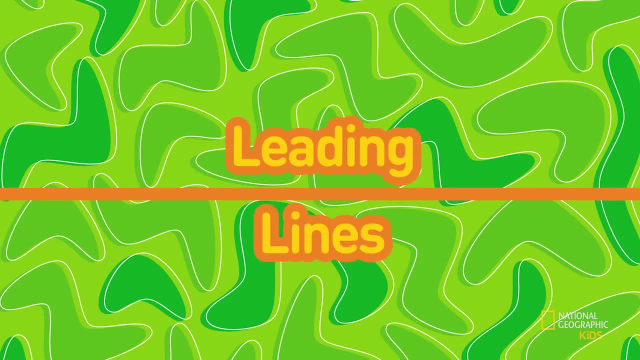 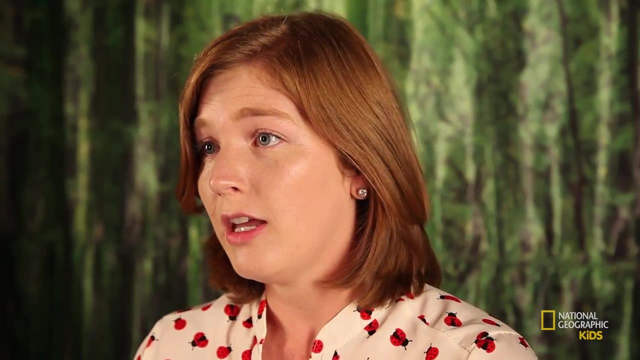 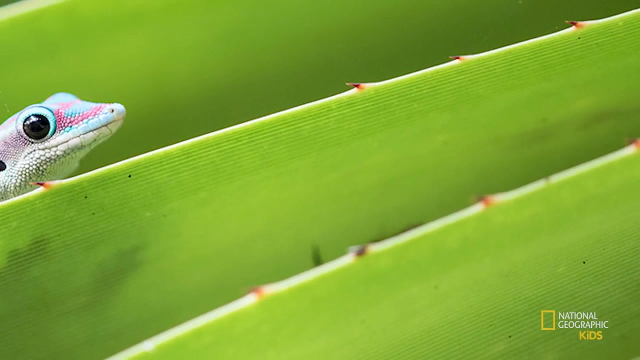 makes you stop and look more closely. Leading lines: Use lines to draw your viewer's eye into the photo. Leading lines can be formed by natural objects such as a river, a row of tree tops, birds of formation, turtles on a log or even clouds. In Gabby's photo, the diagonal lines created by the plant lead. 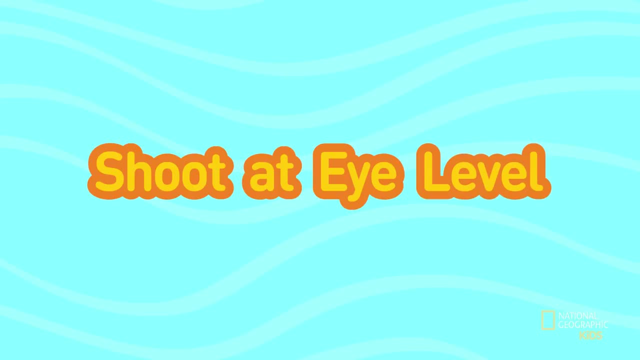 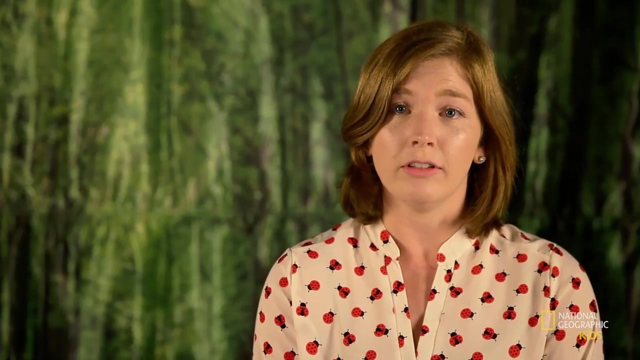 your eye right to the cute little gecko. Shoot at eye level. Instead of photographing an insect or your dog from above, get down on the ground to their eye level. Photos are more compelling when your subject is looking right at you. This grasshopper was sitting on a leaf about two feet off the ground. Instead of photographing, 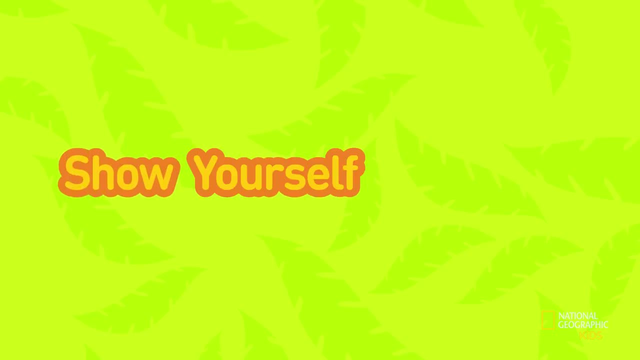 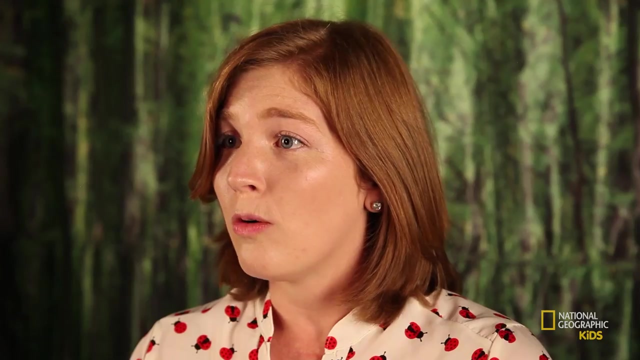 from above. she got right down to eye level. Show yourself in nature. Be creative in how you shoot your photos. You can photograph your friend silhouetted against the sunset, or get close and focus on little details, like your friend planting vegetables in the garden. 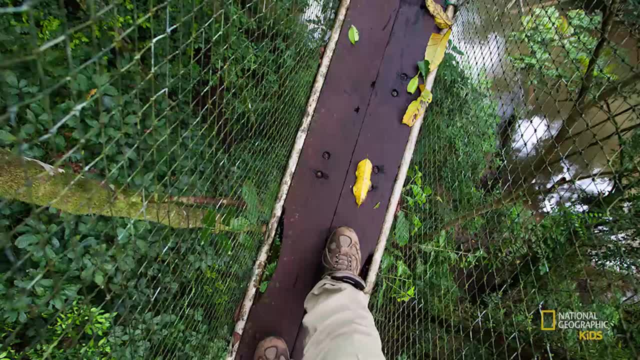 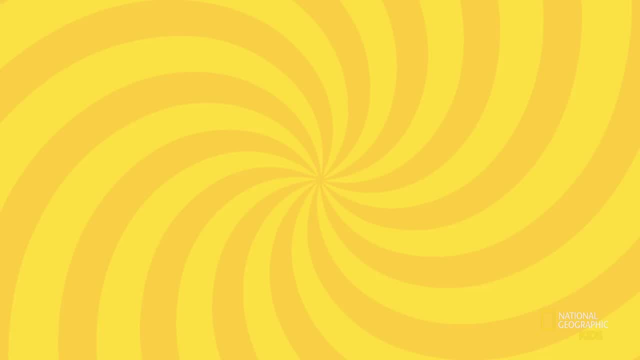 Show us why you love nature. Gabby wanted to show how far above the ground she was, so instead of photographing off the side of the walkway, she chose to photograph her feet. Experiment. Experiment with different angles, different lighting and different techniques. 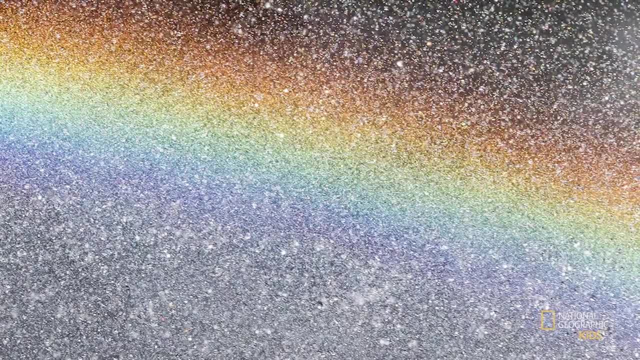 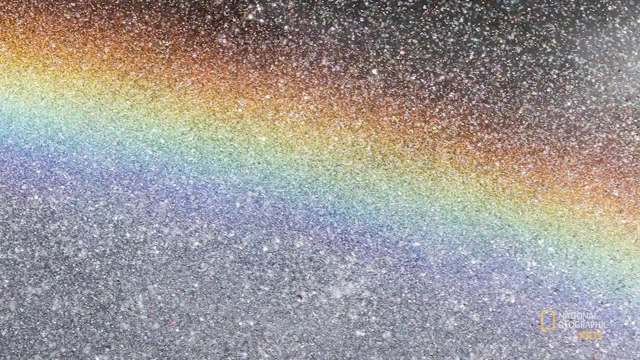 Be creative and have fun. Instead of photographing the entire waterfall, Gabby zoomed in to focus on the rainbow created in the spray of water. She experimented with many different compositions before choosing this one. Check back at natgeokidscom for a gallery of her favorites. 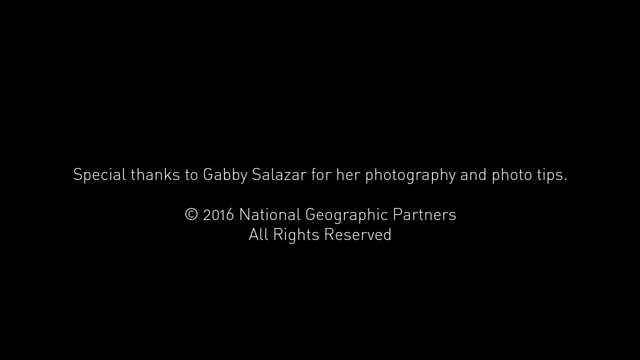 If you enjoyed this video, be sure to like, comment and subscribe for more like this.